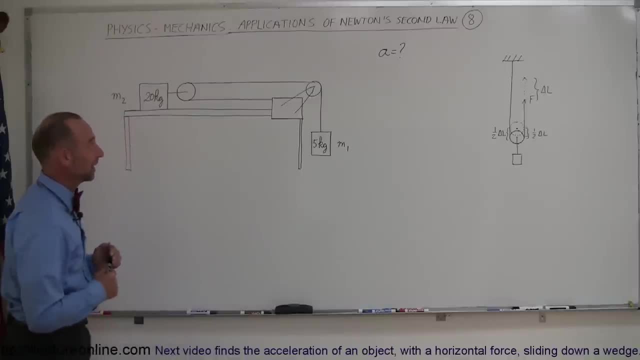 And here's a very interesting example. that's a good application of Newton's second law. We have a table. On the table we have a heavy mass, mass 20 kilograms, attached to a pulley like this. We have another mass, a small mass, right here. 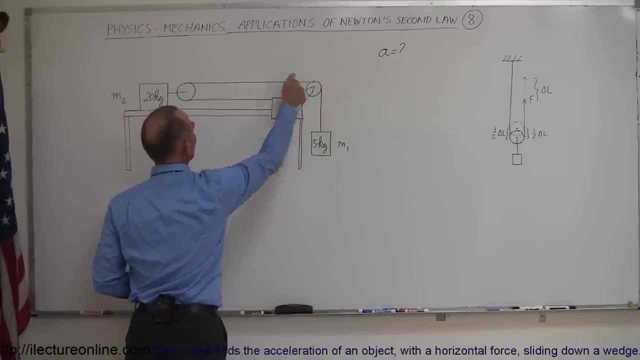 attached to a pulley like this- This single string goes across this pulley, around this pulley- and attached to a block which is attached to the table. Now you can imagine if there's no friction here. so let's say mu equals zero over. 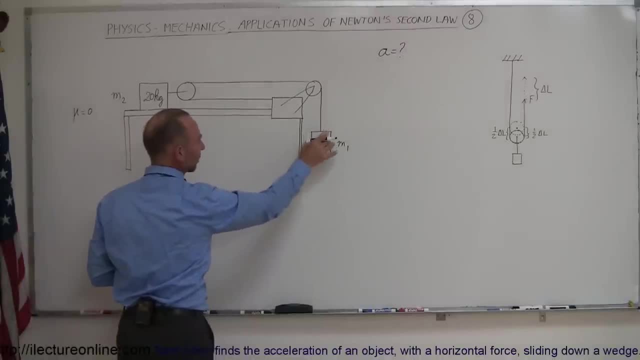 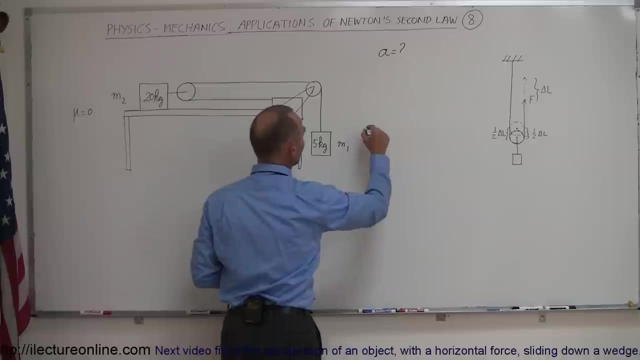 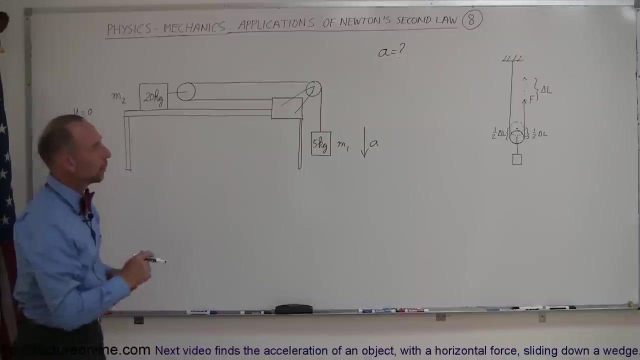 here, between this mass and the table, that this mass will begin to accelerate downward, which means that this mass will begin to accelerate to the right. And so the question is: what is the acceleration of this five kilogram block downward? And let's see what is the tension in the string. So let's say this is tension one. 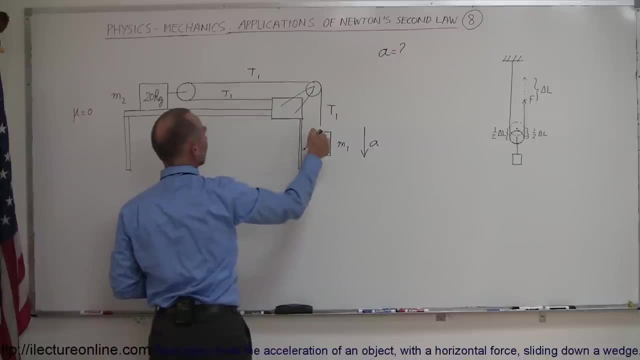 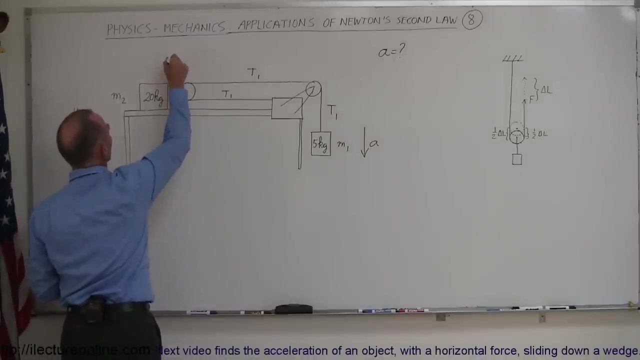 Let's call this tension one. Let's call this tension one because this is a single string. The tension should be the same everywhere along this string, assuming that these two pulleys have no mass- negligible mass, of course- and no friction. But what about this tension right here In here? let's call this: 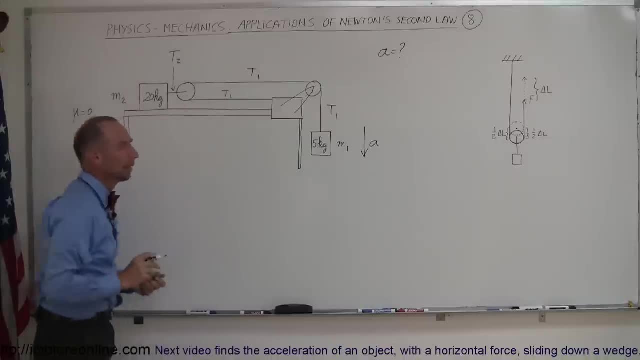 tension two, because that is not equal to tension one. How do we know that? Well, let's take draw a free body diagram of this pulley right here. We notice that these two tensions will be pulling to the right and this tension will be. 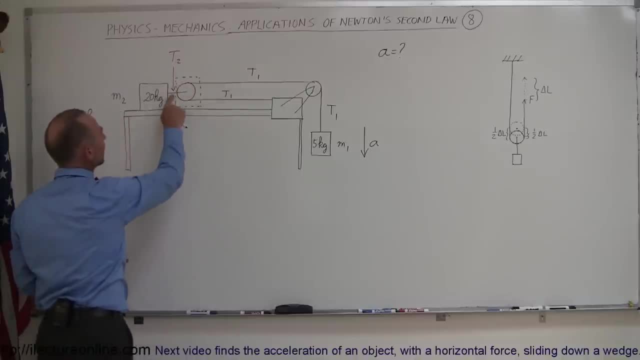 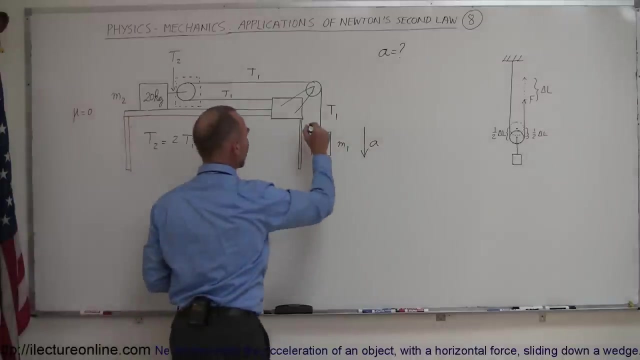 pulling to the left, Which means that this tension must be equal to both of these tensions right here. or we can say that T2 is equal to two times T1. So there's definitely a relationship there. Let's take a look at this over here. Let's draw a free body. 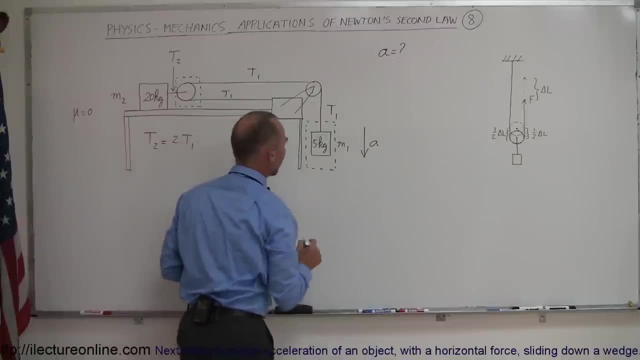 diagram right here. We can probably say here that tension one is going to be equal to the weight of this object. Remember, this is going to have an m1g downward, like this. So that means that the tension will have to be equal to the m1g, the weight of the. 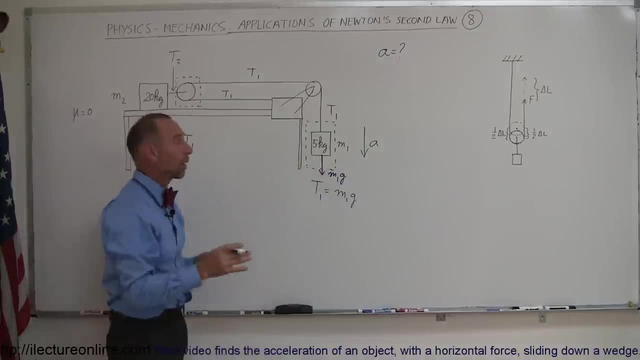 object: plus or minus the force required to accelerate this. Now, since it's accelerating downward, it's going to be minus m1a, And since we have T1 being half of T2, or T2 being twice T1, we can say that whatever the tension is right. 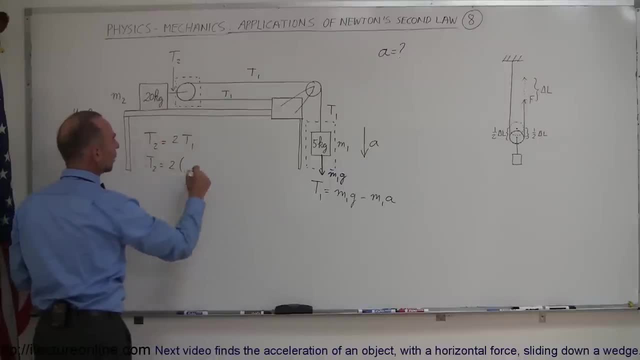 here, T2 can be set to be equal to two times T1, which is m1g minus m1a. All right, so we have a relationship there. Now also, what I can say is that whatever the acceleration is of m1, the acceleration of m2 should be half of. 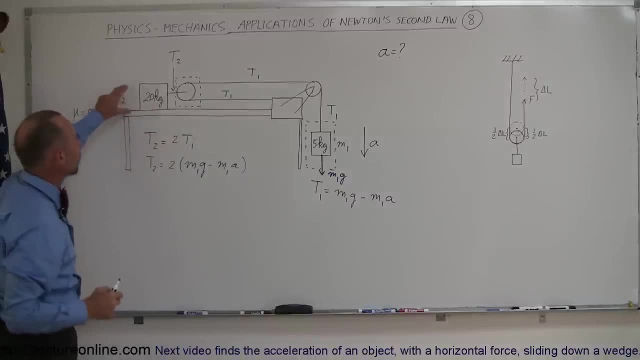 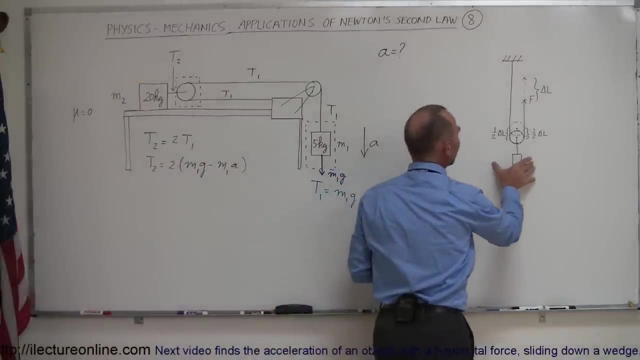 that? Why do I say that? Why will this block move at half the acceleration or half the speed of m1?? Well, to help understand that, I have this little drawing right here. Let's say we have kind of a similar situation. We have a rope attached to the. 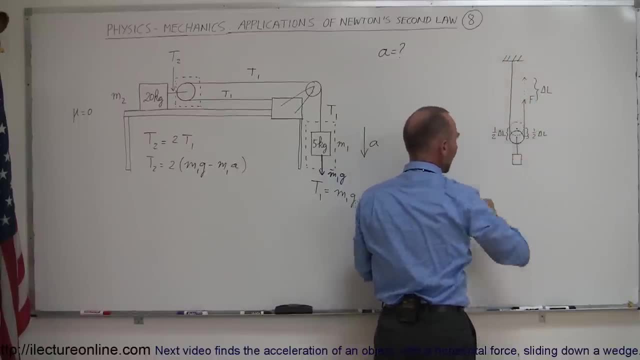 ceiling coming down around the pulley, the pulley- we have a mass- let's call this mass m- attached to this pulley right there now. if i pull on the string on one end right here and lengthen this by delta l, if i lift this up a distance of, 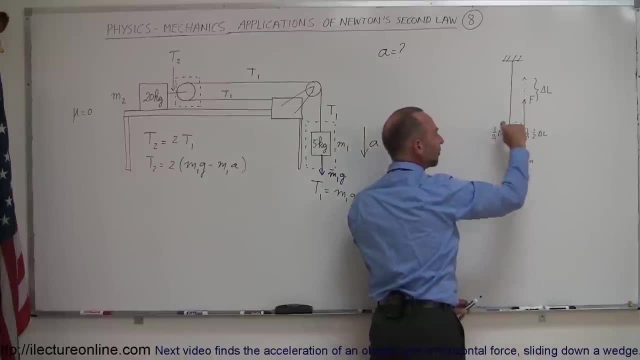 delta l notice that the pulley will only go up about a half a delta l- not about, but exactly half a delta l, because this delta l is accounted for in a piece on this side of the pulley and a piece of string on this side of the pulley. so if you add these two up you'll get a total of a half. 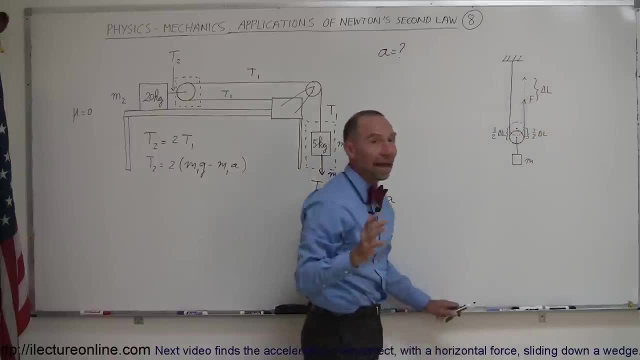 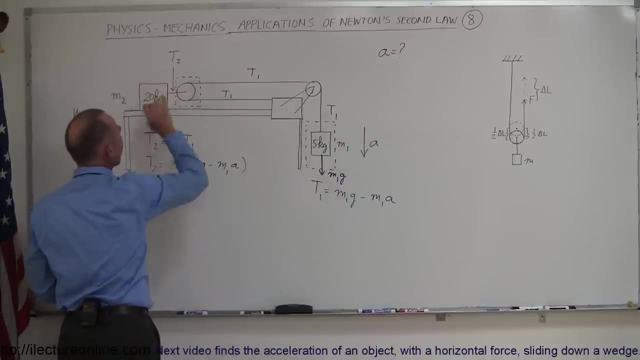 of a full delta l, which means that the pulley only moves up a half a delta l. so same here. when this drops a certain distance, let's say delta l, then this mass will only move to the right at half a delta l, which also means that whatever the acceleration is for this mass right. 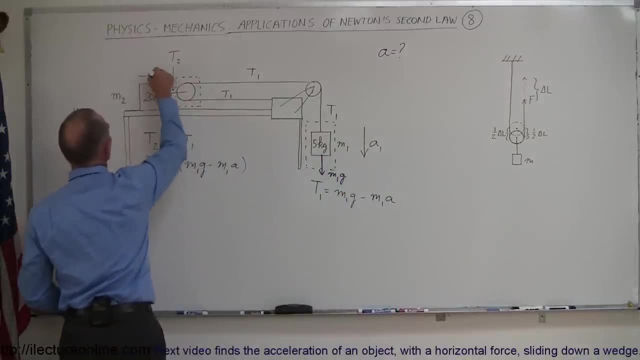 here. so i call this a1 and i call the acceleration of this one a2. i can then say that a2 is only half of a1. all right, so here's a relation between the accelerations of these two blocks and here's a relationship between the tension on this string versus the tension on that string. 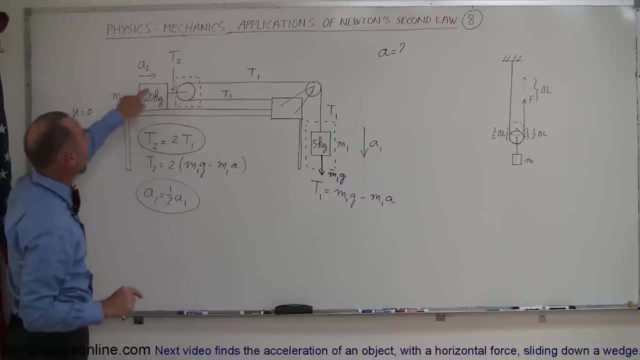 now also see that this tension right here will cause this block to accelerate. so using newton's second law we can say that f equals m, a and so the on the 20 kilogram block that the f is the tension right here. so we can say tension 2 is equal to the mass of that block which is in. 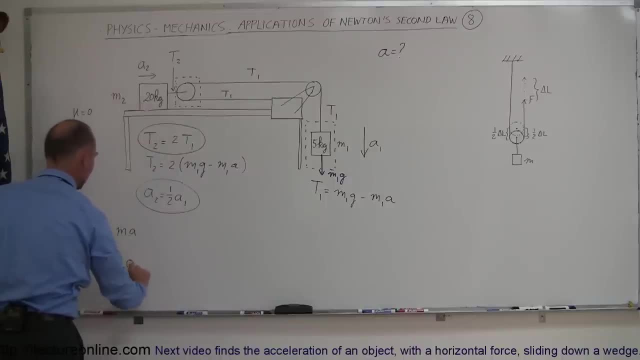 this case m2 times the acceleration of that block, which is a2, and over here i have tension. 1 is equal to m1, g minus m1a, and i know that this is related. a2 is related to a1 like this: now, if i put it all together, i can say that t2 is twice t1. so i 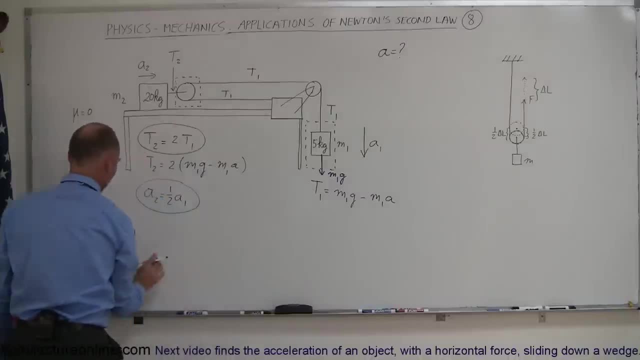 could say that this is equal to twice this. so m2 a2. so i can say that m2 a2, which is equal to t2, is equal to two times t1, which is m1 g minus m1a, m1 g minus m1a. and finally, since a2 is half, 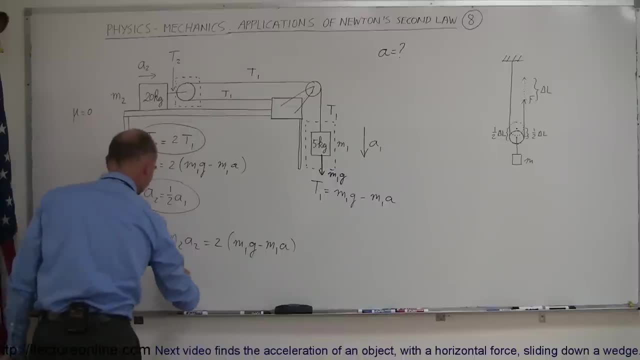 of a1, i can replace a2 by half a1, so i could write that m2 times one half a1 is equal to two times m1, g minus m1a. and now i have a single equation with only unknown in it, which is acceleration. wow. so i used the concept that t2 was twice t1. 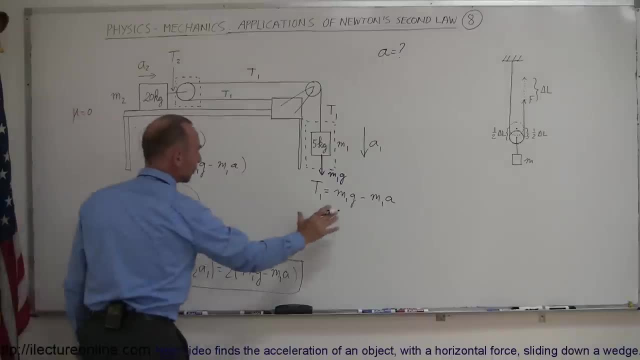 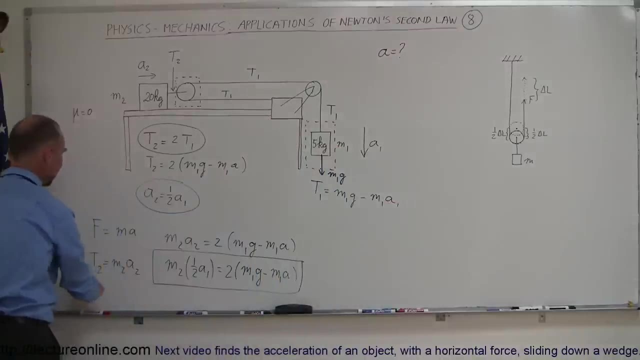 and that a2 was one half a1. and then i solved for the equation where t1 was related to the acceleration- i guess this would be a1 of this block right here- and t2 is related to the acceleration of block number two- then i can combine the two equations and i have a single equation with just 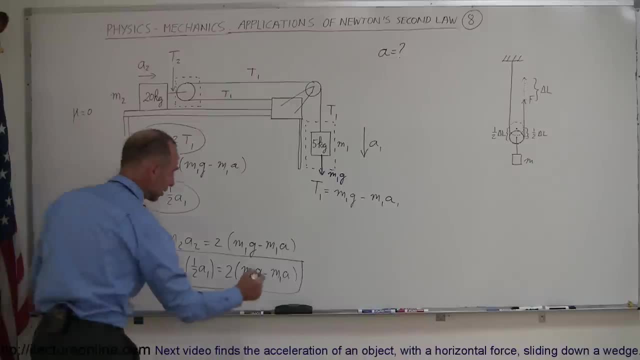 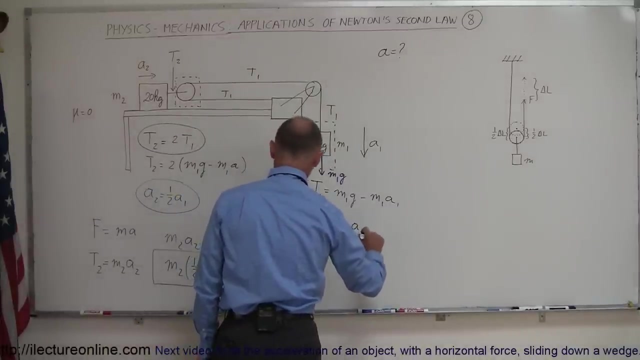 the acceleration in it. so now i just have to solve for acceleration one, so i can call this, i guess, acceleration one. all right, so how do i do that? hmm, how about if i multiply both sides by two to get rid of one half? so now i have m2. a1 is equal to four times m1, g minus m1a, so i can go. 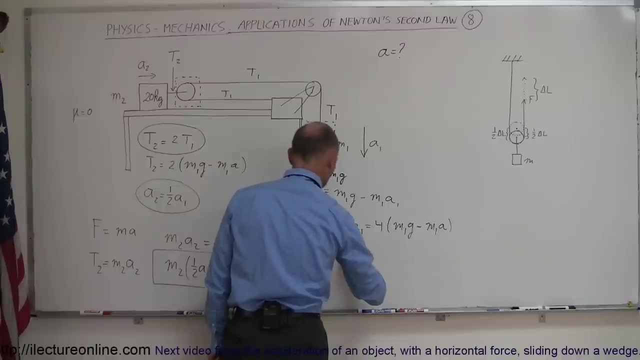 ahead and multiply that through to get rid of parentheses. so m2 a1- call this: a1 is equal to 4 m1 g minus 4 m1 a1. now i can go ahead and move this over to the other sides. so we have m2 a1 plus 4 m1 a1 is equal to 4 m1 g. then i can factor out an a1. 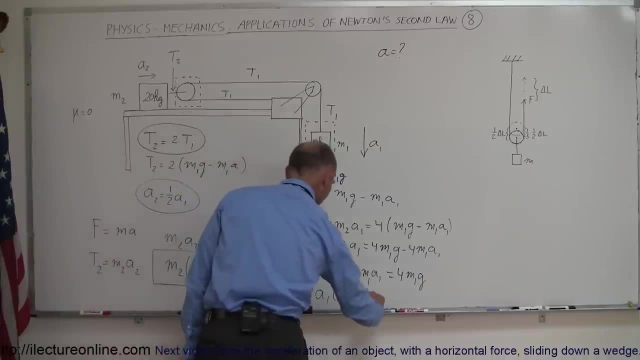 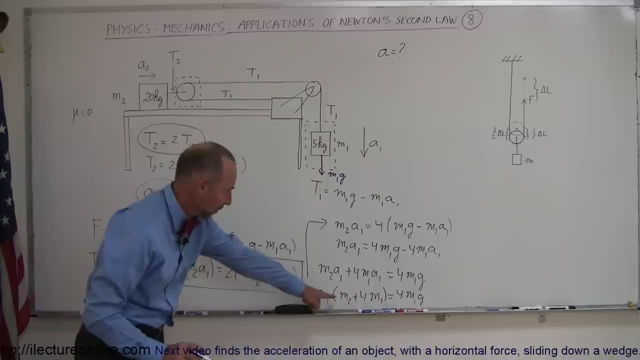 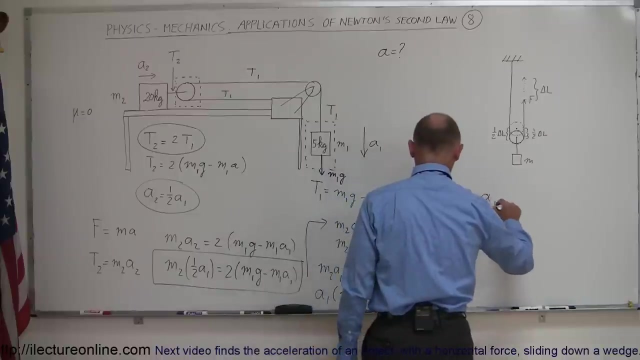 so i have a1 times m2 plus 4 m1 is equal to 4 m1 g. and finally i can divide both sides by m2 plus 4 m1 and isolate a. so i'll need a little bit more board space. so i now have a1 is equal to 4 m1 g. 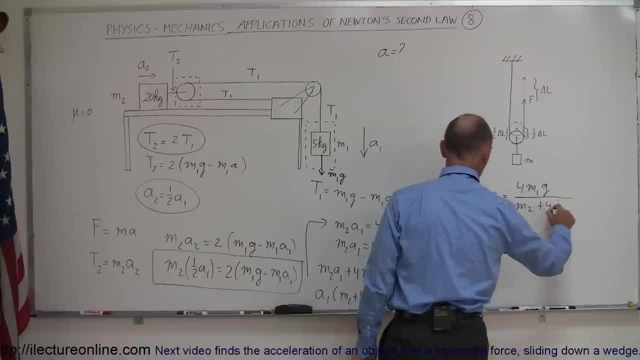 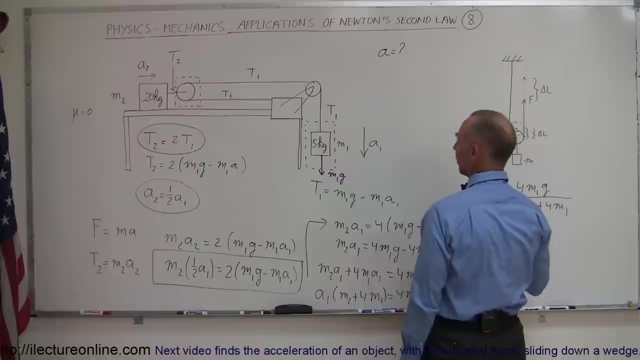 divided by m2, plus 4 m1, and i can go ahead and just plug in all the numbers that i know. let's see: m1 is 5 kilograms, so i have 4 times 5 times 9.8 divided by m2, which is a 20. 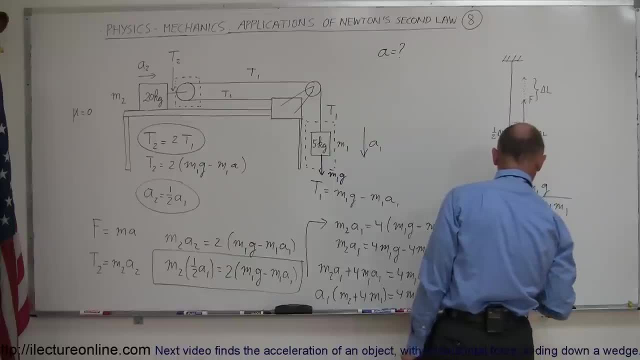 plus 4 times m1. 4 times 5 is 20 as well. that would be 40, and so let's go ahead and do that's 20 divided by 40 times 9.8, which is 4.9 meters per second square. so that would be a1. so here we have. 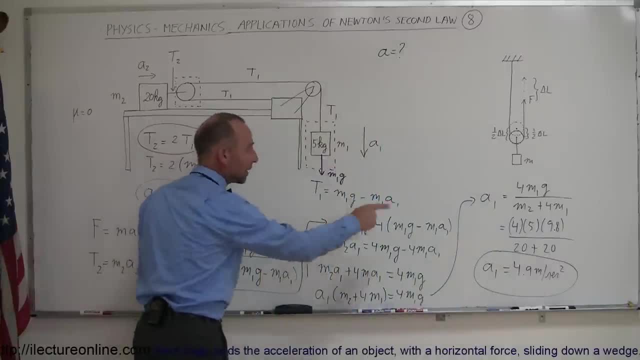 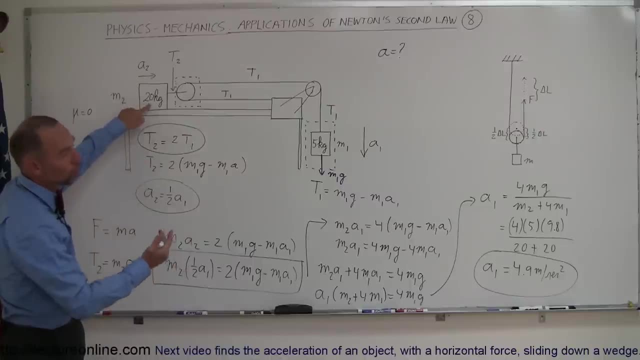 found the acceleration of the five kilo kilogram block to be 4.9 meters per second square, which means that the acceleration of the 20 kilogram block would be half that, or two point four, five meters per second square. wow, that was an interesting problem. and again the concept. 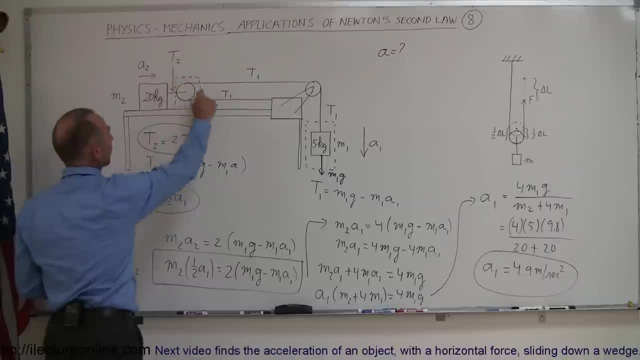 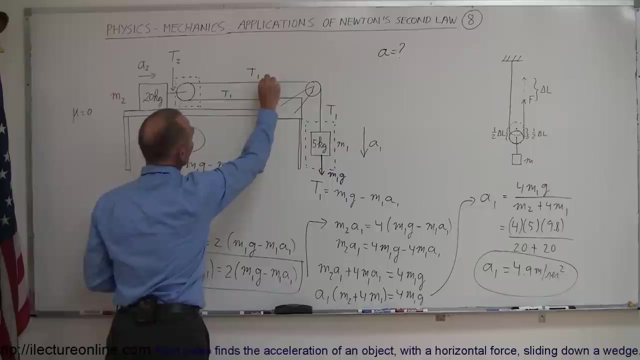 is that if we draw a free body diagram of this pulley right here, we can see that both of these tensions add up to this one tension over here, which means that t2 is equal to two times t1. also, we know that as block, the five kilogram block moves this way and therefore pulls on the 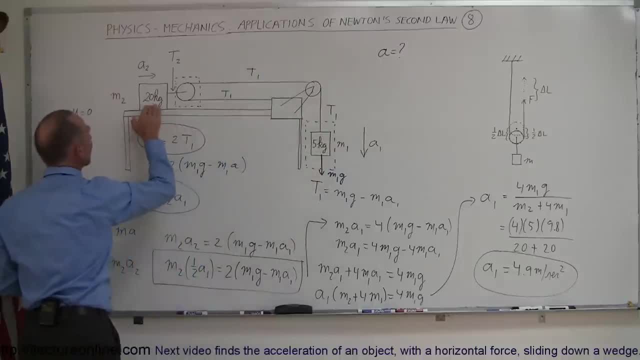 string that whatever distance this one covers, this one covers only half the distance. so whatever the acceleration is of this block, that means this block only has half the acceleration. so we have that relationship right there. then we use newton's second law on both sides. we use it here on the left. 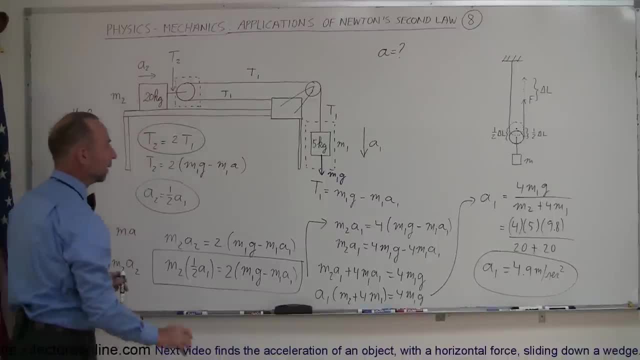 side f equals ma, which means t2 equals m2- a2, and over here t1 equals m1 g minus m1 a. then we can set those two equal to each other. actually, this one t2 will be twice this one. we end up with a. 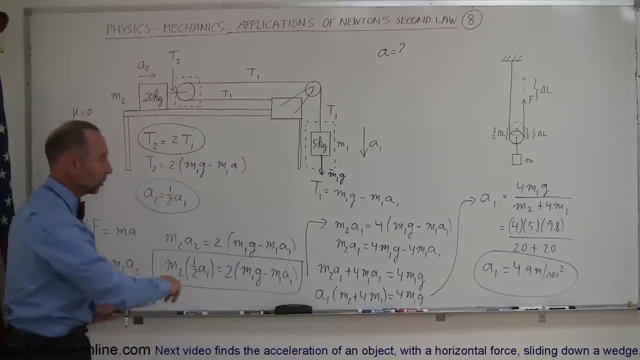 single equation with just a1 in it as a single variable, which we then algebraically solve. and we solve and voila, we got the answer all right. a little more challenging, but that's how you do that.